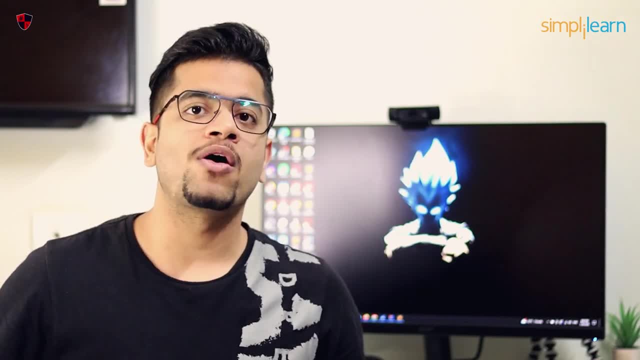 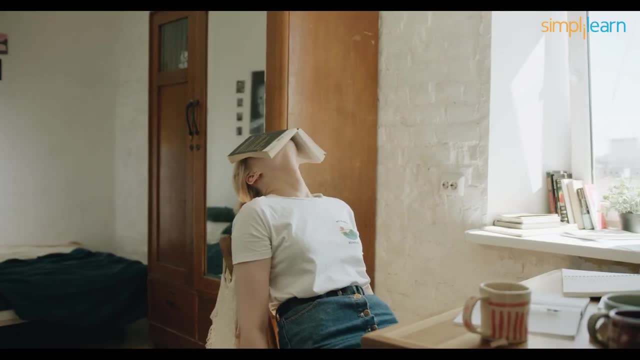 for learning. Why do certifications? Why not degrees? Why not colleges? So the fact is that college learning is not many times, not very often, at par with what industry demands. There is a huge gap. You may not even be able to learn cybersecurity in 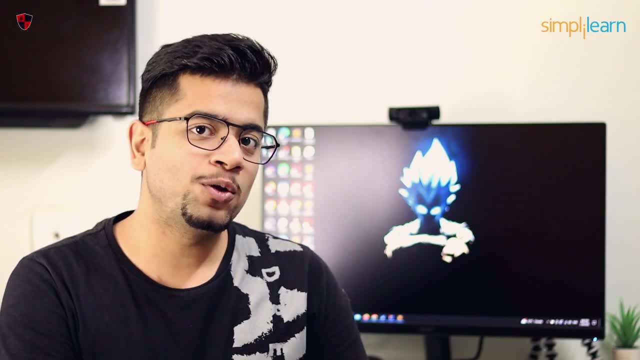 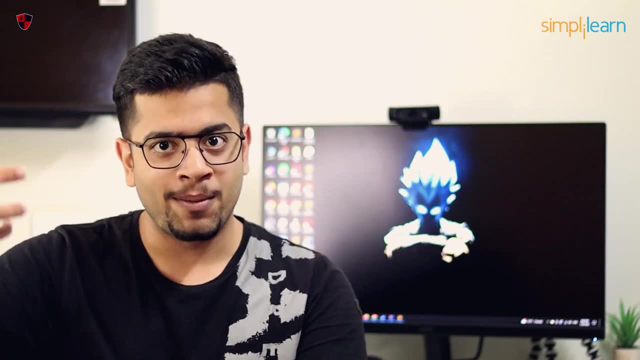 your college studies. That's the truth. But in order to be good in this field, you need to be adaptive. You need to adapt at a pace that's not very often kept up in college degree programs. Syllables don't very often change in. 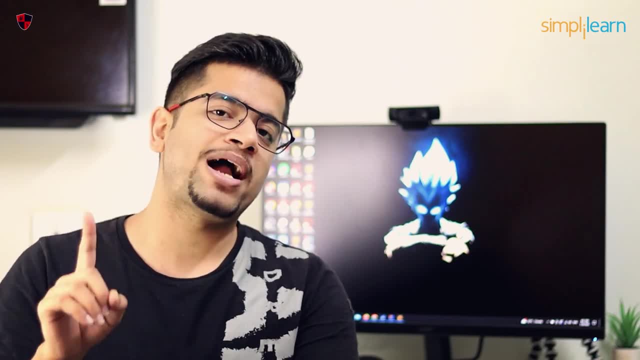 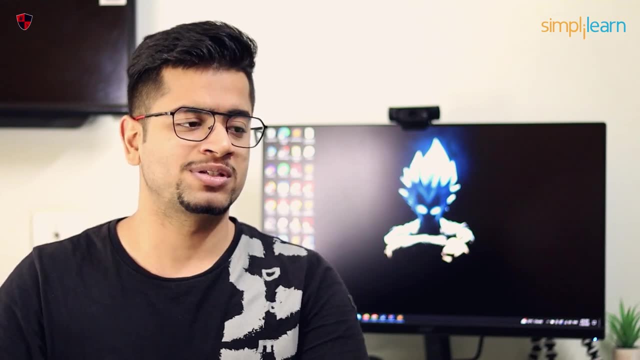 this degree programs, While I do recommend people to get at least one bachelor's degree in CS or IT, but certifications are the best way to boost your resume and skills at the same time, because they take very less time. They just focus on one important niche and go very deep into it. 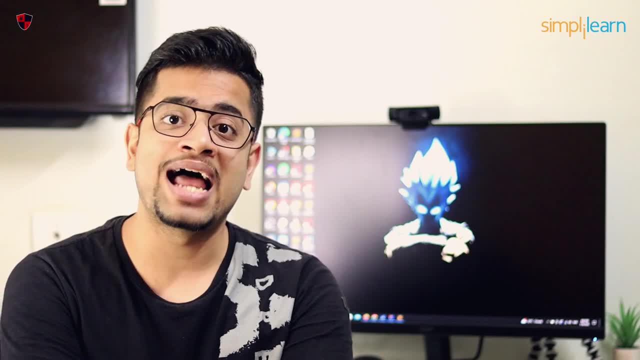 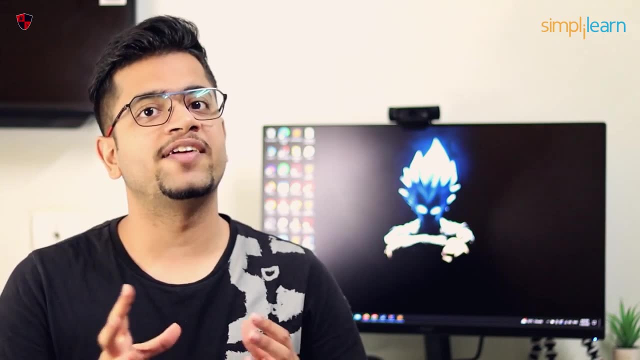 And they generally don't cost you as much as a degree, While degree can cost you- in lakhs maybe 10 or more, but a certification will not cost you more than a lakh or two, And in a degree you're taught many more things that you don't even need in your career, that you want to pursue, But a certification will give you a path to follow in your future. So here are my picks for the top five certifications in cybersecurity that will give you a good position in top company and your dream job. So I'll try to list them. 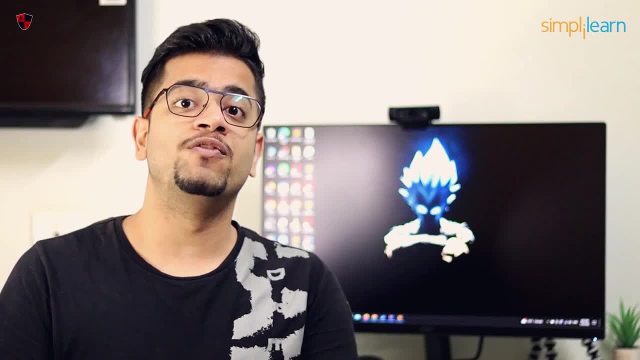 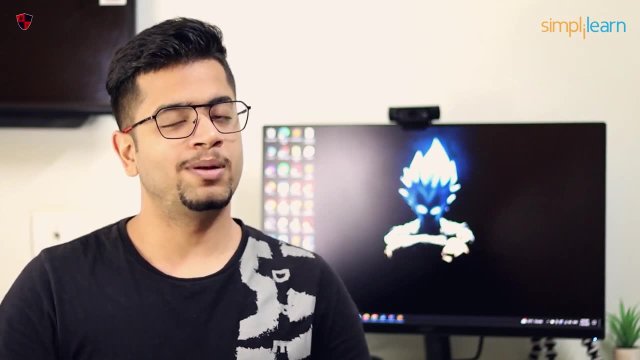 in order of the experience level. So the very first certifications that you will and you should do is CEH: Certified Ethical Hacker. This is the most basic course that you can do. that will build the very fundamentals of you understanding how attacks work, how to find issues. 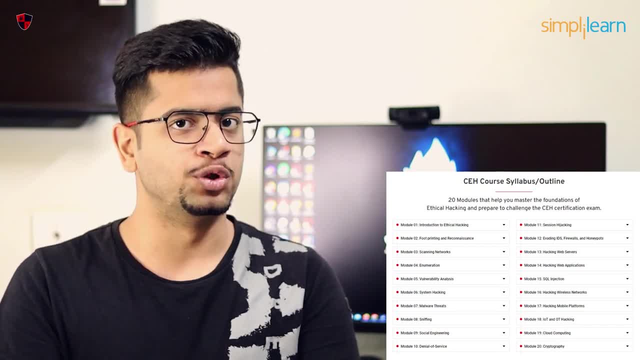 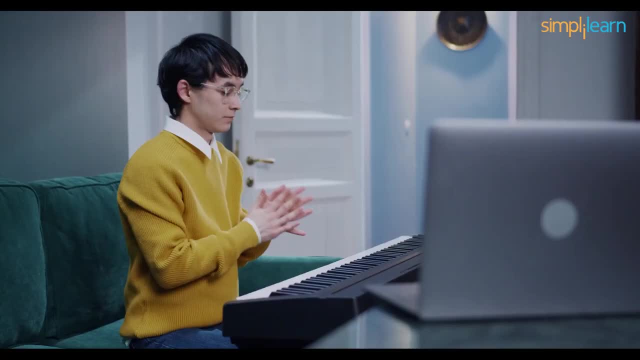 in hacking a system. This is the bare minimum that everyone should do in order to get started, to get to know what this field looks like. So people new into this field and just want to start their career as a fresher, I think this is one of the best certifications to do. I know many people. 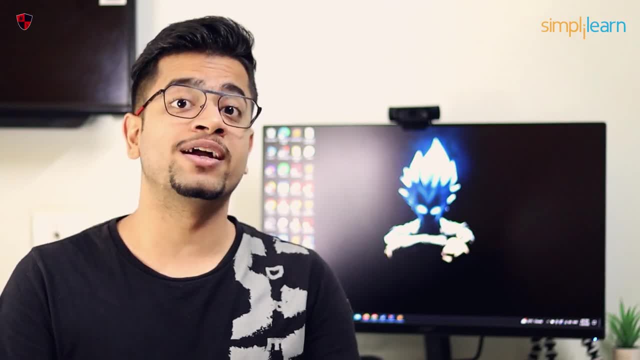 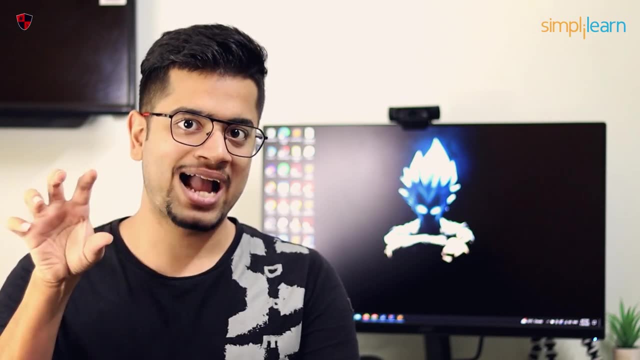 count it as worth because it's lacking very hands-on training on real world scenarios. But at the end of the day it's a building block and it gives you a mark of a certified hacker. And still, HRs in India look for this badge at the bare minimum in many cases. 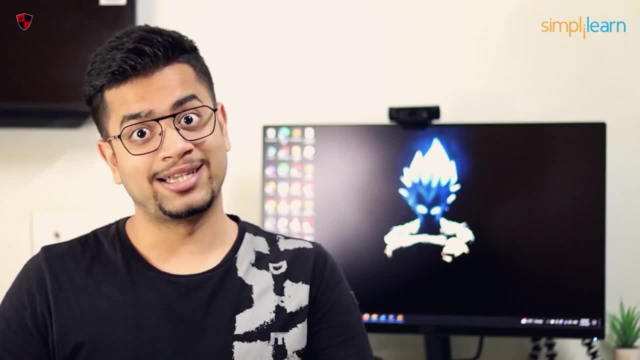 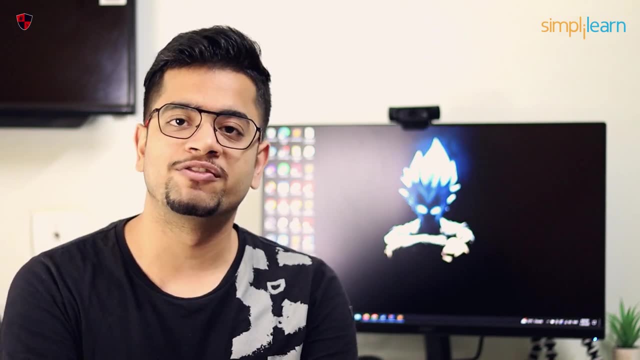 So you can be hired as a pentester or a security analyst and then break the barrier of experience once and for all And while you work you can focus on your skill set and build and do more certifications in the future and just keep growing. I know it's difficult to manage skilled 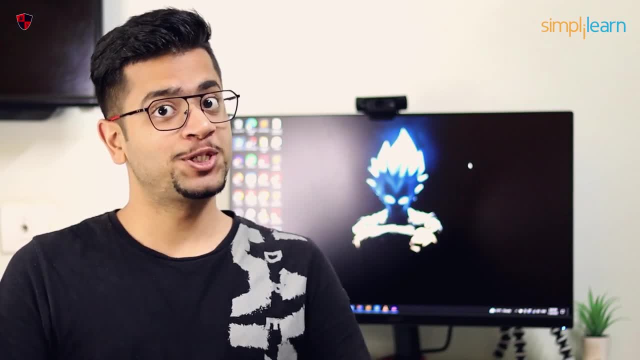 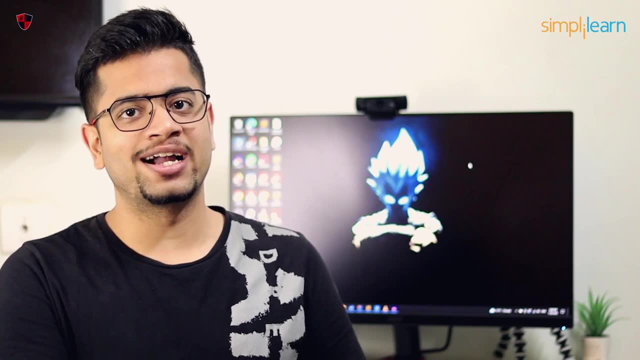 development when you work full-time. Even I face the same, especially when you are doing it on your own in self-learning. Well, well, well. I know a program that can make you a certified ethical hacker while you study and guide you on your learning. I'm talking about Simply Learn's. 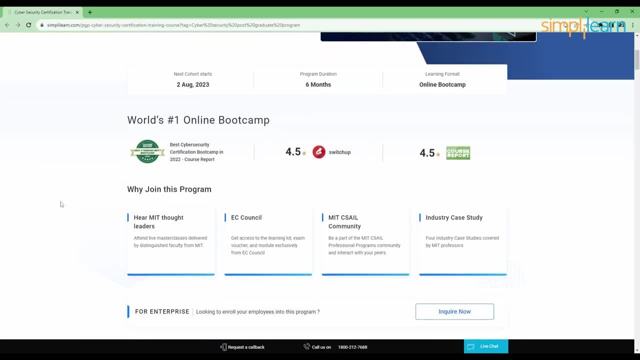 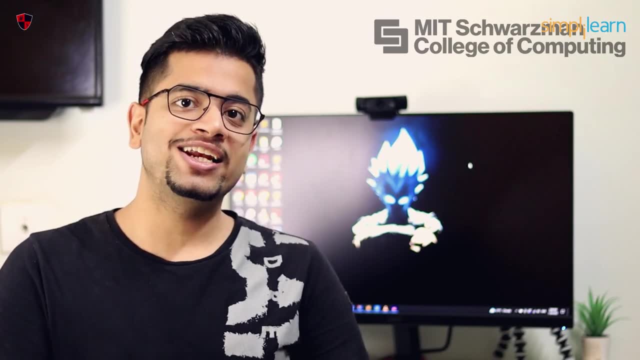 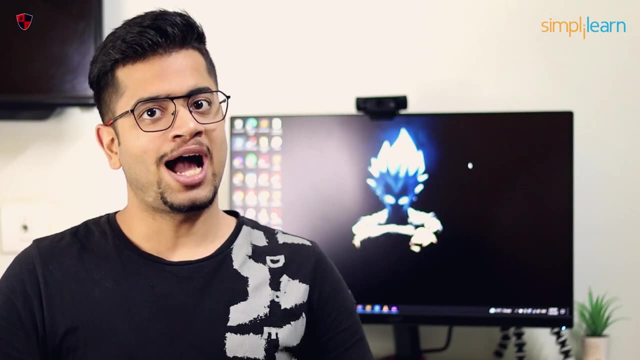 postgraduate program in cybersecurity that is backed by top expert study programs and faculty from MIT, Schwarzman College of Computing and even EC Council. The program is an online bootcamp that is a six-month course where you will learn from industry experts how to design build. 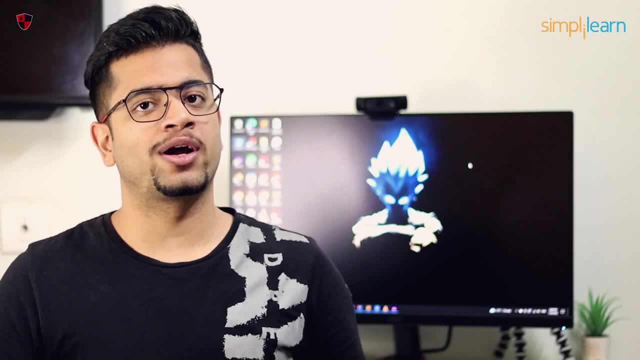 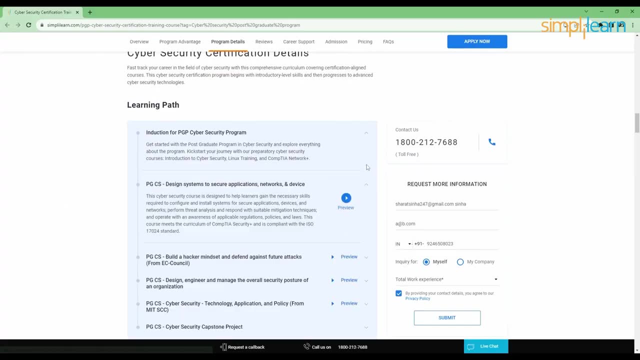 and implement secure systems at scale in large-scale organizations. The course covers 20 of the most popular and important security domains and how to apply best practices in all of them, And it is also aligned with CompTIA Security Plus and will teach all the standards. 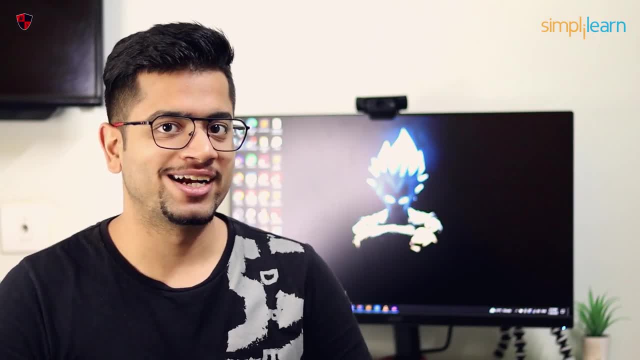 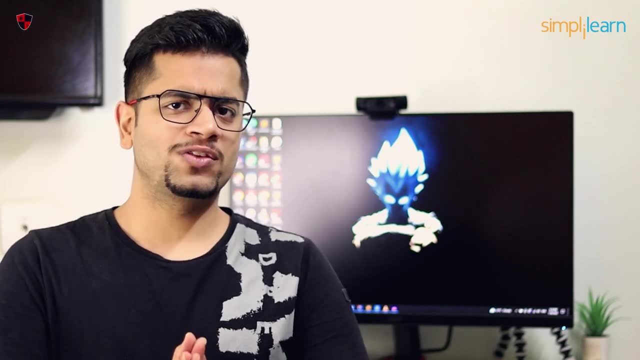 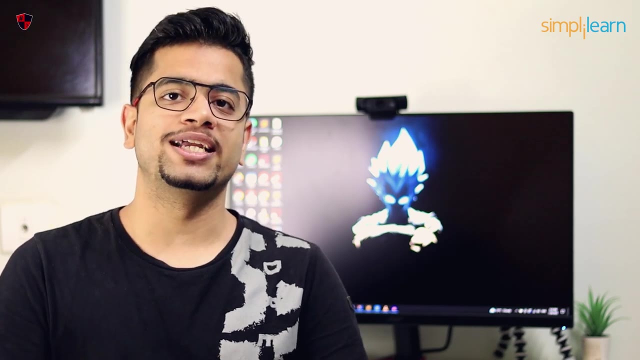 covered there. It will also teach you how to develop a hacker mindset, identify and manage threats, and also the overall security posture of large-scale organizations. At the end of the learning, you will get a capstone project where you will apply your industry skills and you will get a chance to showcase your expertise to future employers. 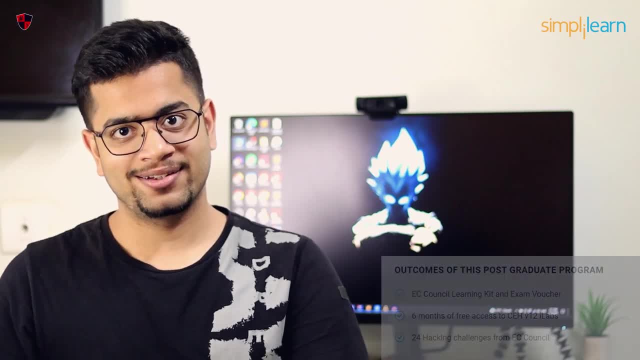 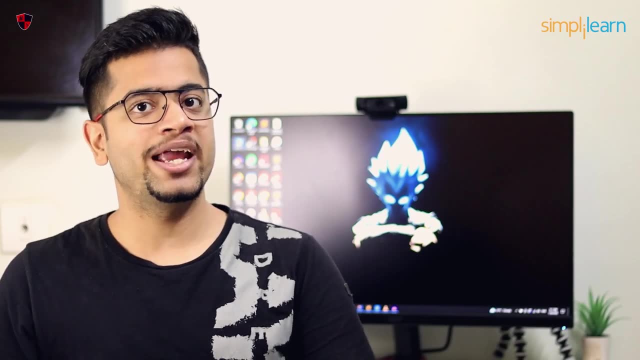 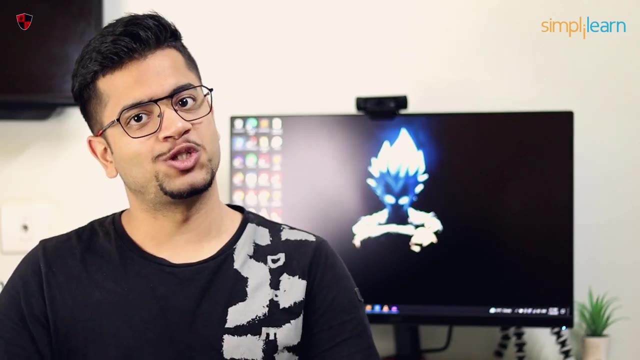 You will also get access to EC Council's learning kit and CEH V12 iLabs access for six months, along with an exam voucher which will make you a certified ethical hacker while you study. And you will also get a certificate from MIT Schwarzman College of Computing. 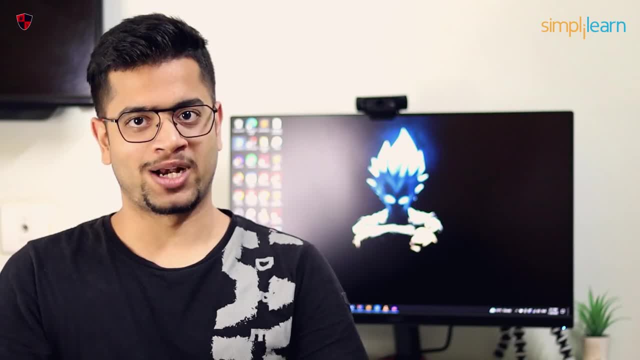 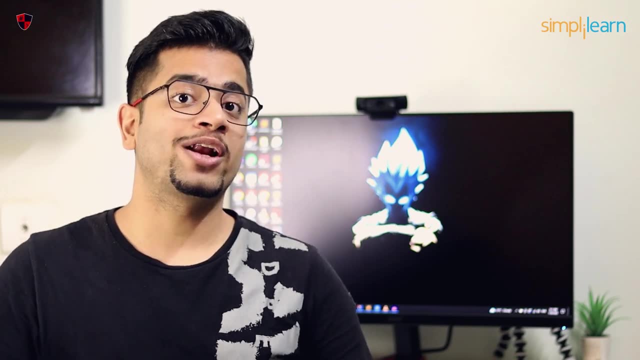 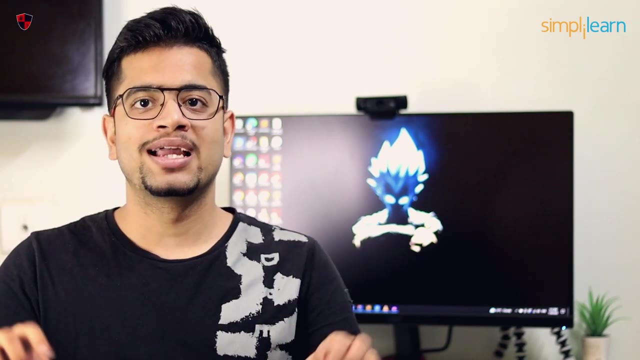 that is really valuable. So to be eligible for this program, you should have a bachelor's degree with 50% or more of grades, and you need not have any programming experience or any prior work experience. So the application for this program is really very simple. Just go to the link in the description. 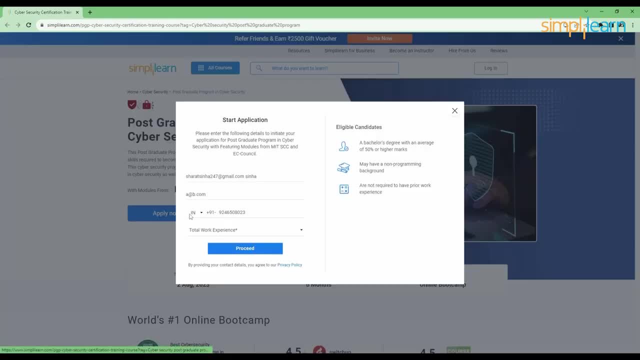 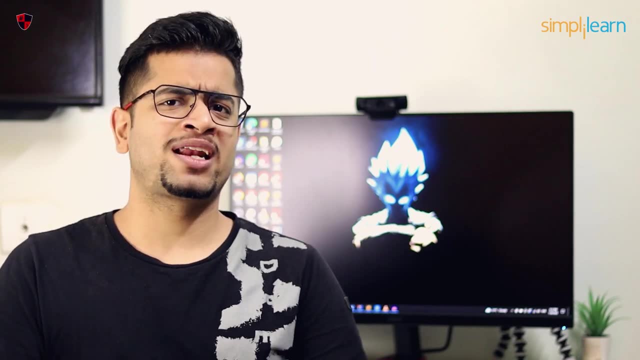 click on the link review all the program details. click on apply now button on the page, fill all the required details asked from you and just submit and wait for the reward back, And I know there are not many good programs out there that can offer you so much. 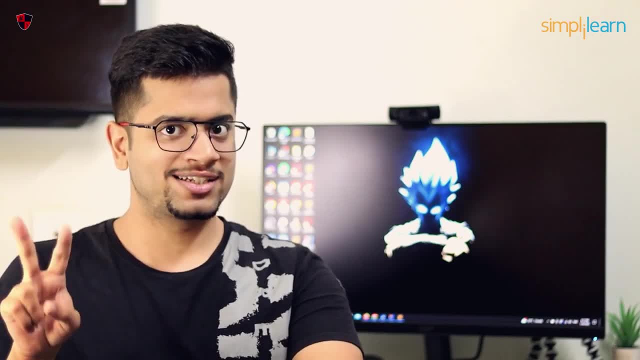 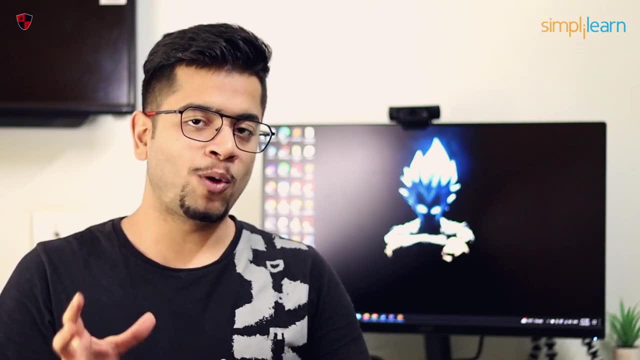 so don't think, just go for it. The second cert is Comtia Security Plus. I know CEH is very popular in India, but if you talk about all around the world, Comtia has done a really good job in establishing a. 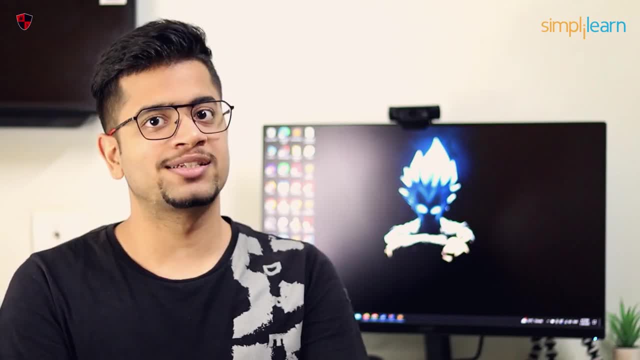 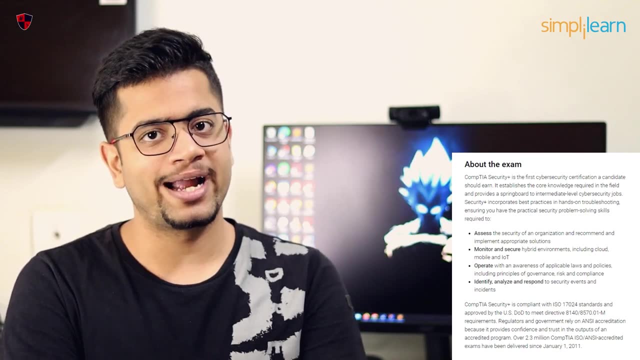 foothold in this industry. This is also a basic certification made for beginners, which will teach you how to secure networks, systems and applications. It's more on the security side rather than the offensive side, And it's greatly aligned to modern enterprise environment and 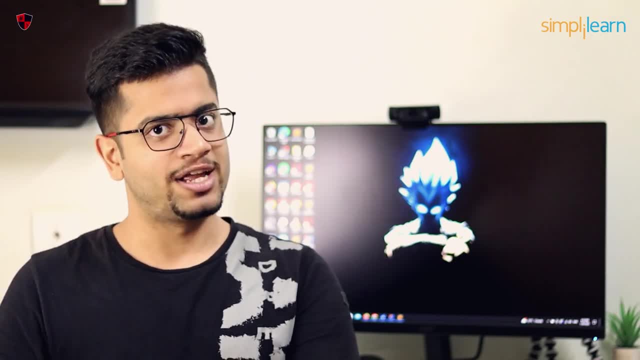 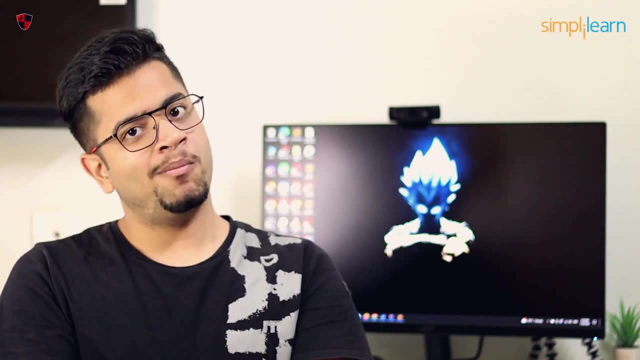 in-demand topics that CEH in itself is very good at, So it's really easy to get started with this. So the third cert is IOT. IOT is a technical certification that in some way fails to cover including cloud, mobile and IOT. It also covers governance, risk and compliance. 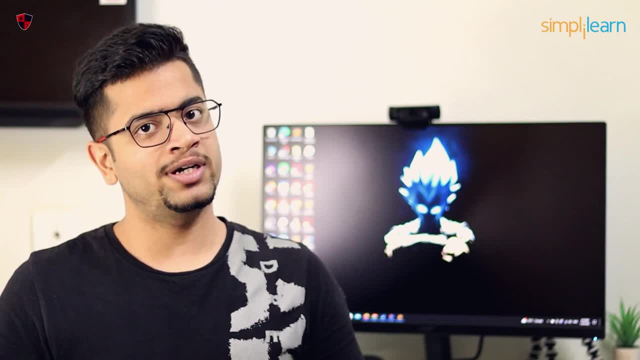 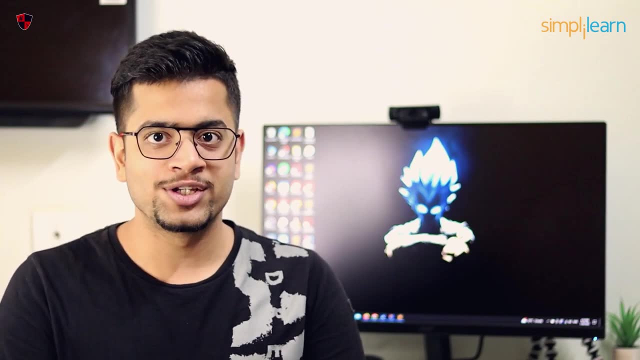 But yeah, many people will think that we still require practical certifications. but this is also a theoretical certification that will have 90 performance-based questions that are not straightforward. that will check your concept overall, what you have learned, but still is theoretical. But if you want to get a job in foreign- in US or in UK- 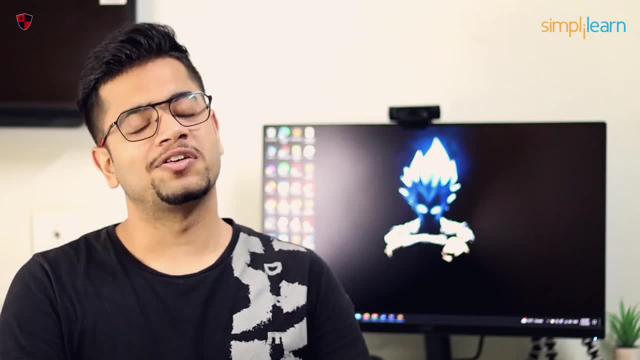 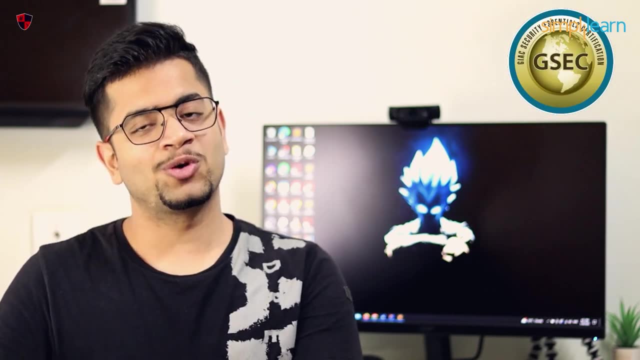 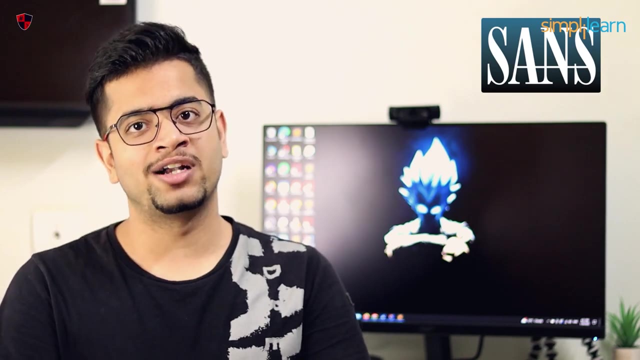 you will need to be a security engineer, a cloud engineer, IT auditor, with a very competitive package. The third one is GSEC or GIAC Certified Security Engineer. Those who are already working in corporate world may already know that SANS is one of the top and one of the best trainers in the 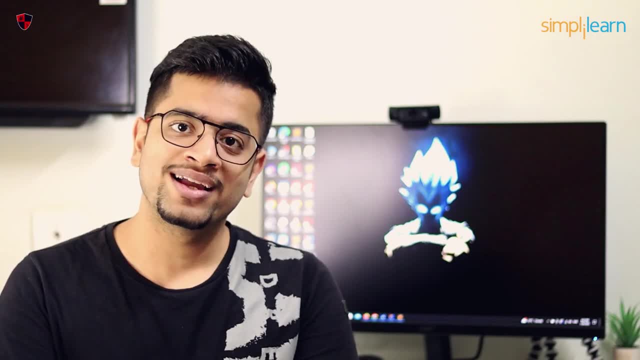 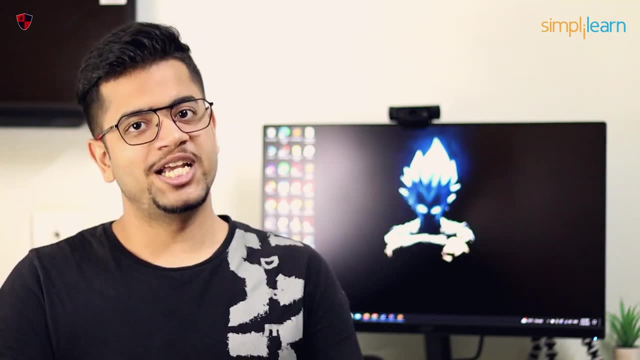 world out there And I've personally done G-PAN and I know that the knowledge that you get there is nowhere else. The top experts from each field come out and teach And of course, that comes with a cost. It is one of the best selling certifications GIAC has to offer. It will teach you active. 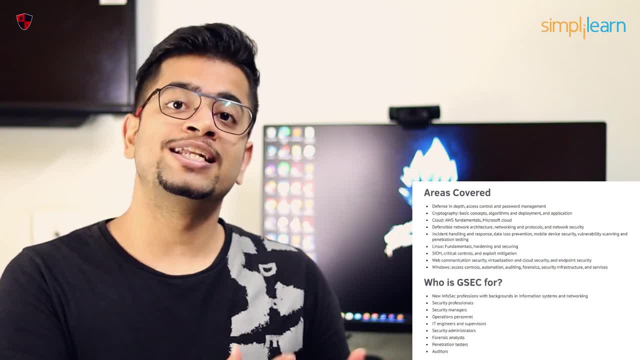 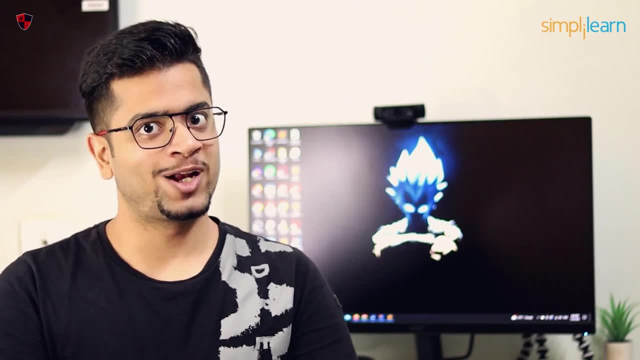 defense techniques, network security, cloud security, incident response forensics. So it is one of the best certifications for blue teaming. And the salary hike here is real. I can tell you from my personal experience if your base is low. 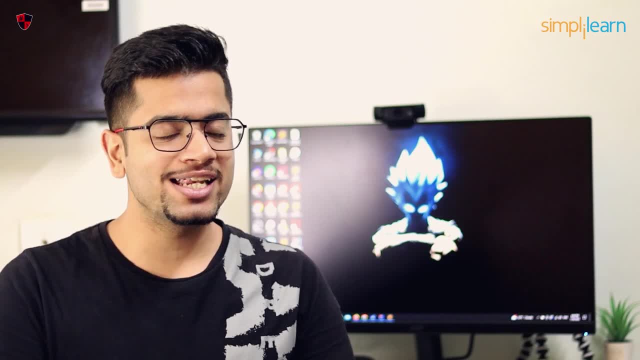 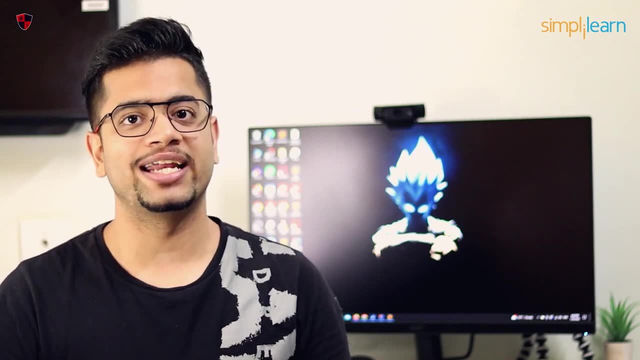 you can easily get a 50% hike. If your base is high, then you can easily get 30-40% hike. But the catch here is I think not many individuals can afford this because the cost is really very high. It can even go to 7-8 lakhs for a single training and certification. So you can only do that if your 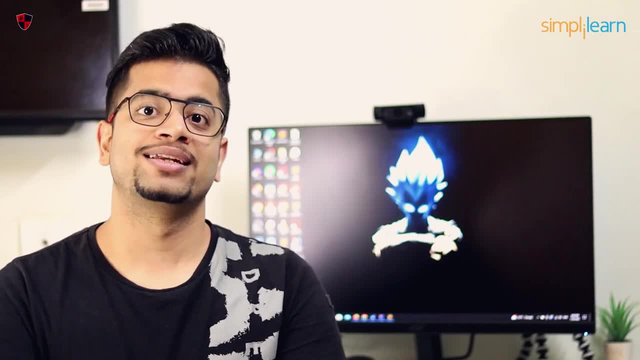 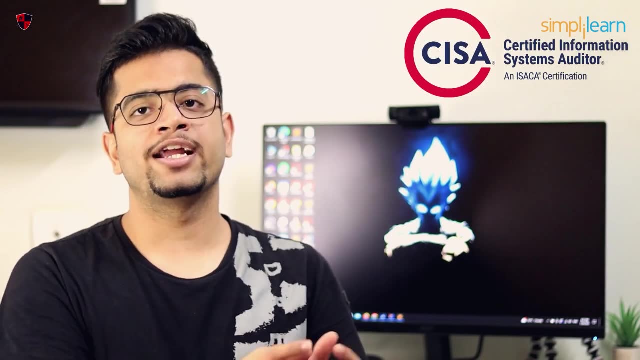 employer sponsors you. So if your employer has a good bank balance and is good enough, you will want to do SANS training again and again, and again. SESA. 4th one is SESA, or Certified Information Security Auditor. Risk and compliance are a very crucial aspect of cybersecurity in today's world, especially if you 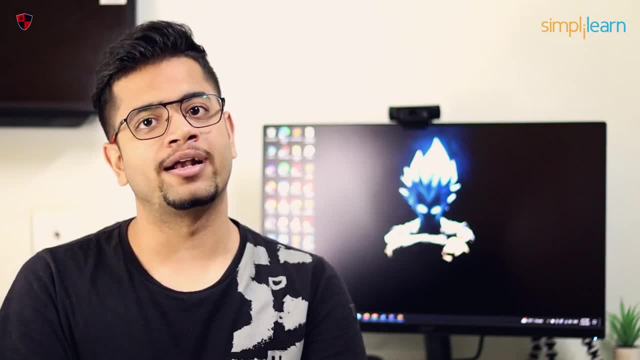 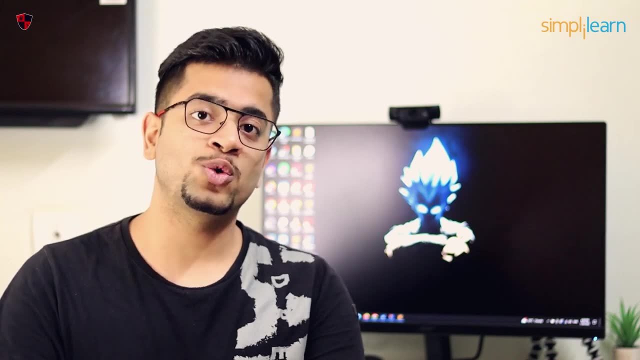 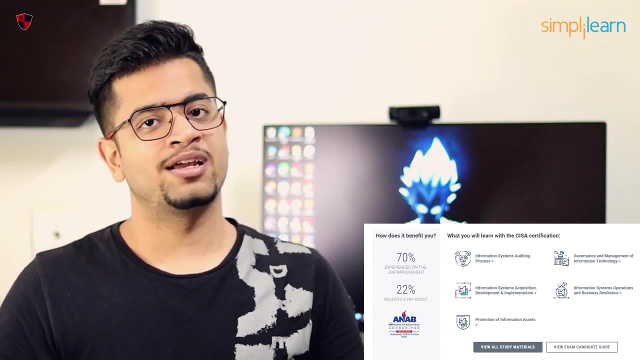 are working in an organization that deals with sensitive customer data, like health, finance and government agencies. ISACA. ACA comes up with this credential that will focus on how to assess security vulnerabilities, how to report and identify risk and manage compliance according to various standards. 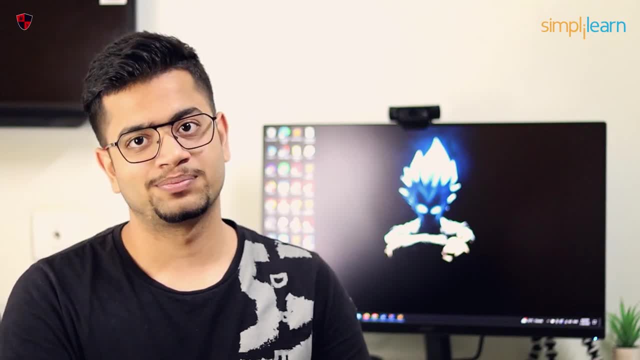 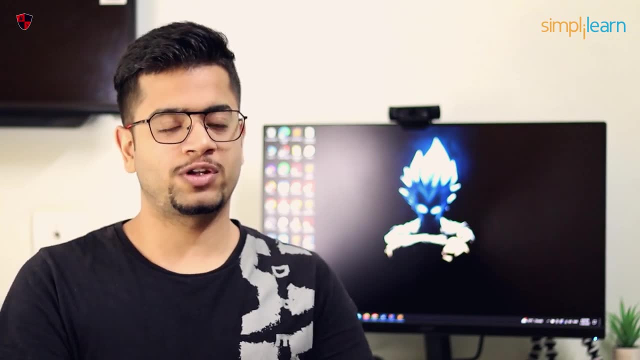 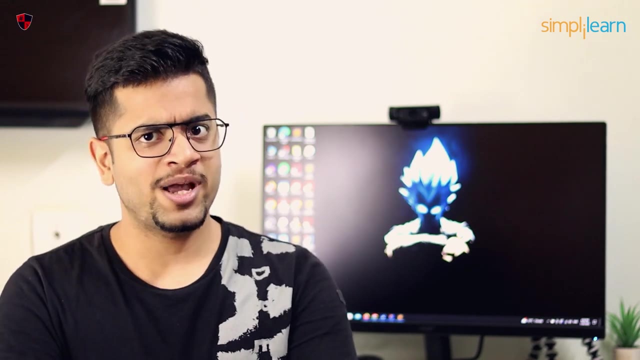 based on the customer data in the department industry they are in. You must have heard about some data standards like PCI, DSS, ISO or HIPAA. They all come around this and this is one of the best certifications that you can do for a governance, risk and compliance job, or a GRC, or an auditor risk manager or a cyber. 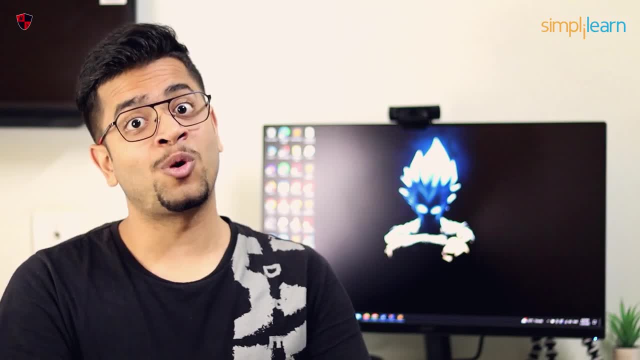 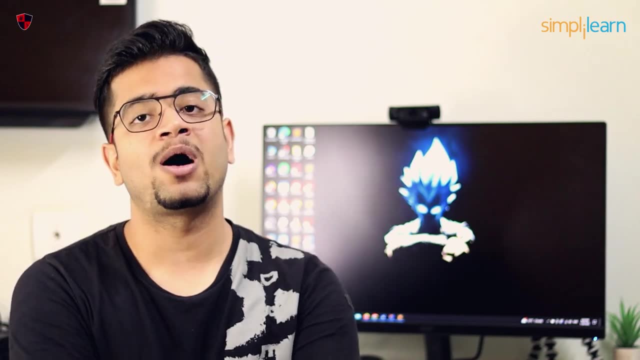 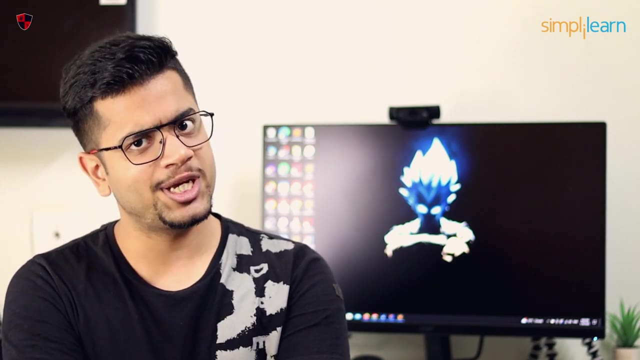 audit manager And the truth is, cyber auditors are more respected than pen testers because they are more wise in decision making and they have a good grip and understanding of how to assess business risk. But this certification requires some prior experience in IT assurance. So if you want to switch into auditing, then you can definitely take this. 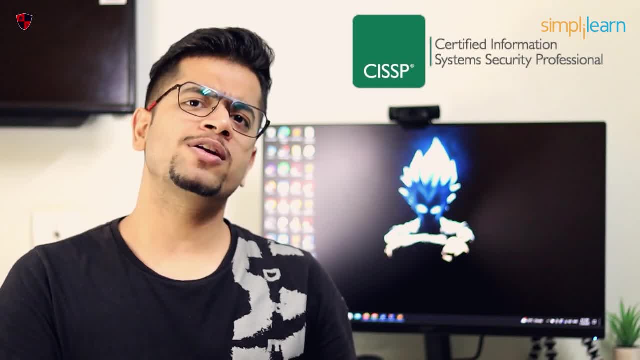 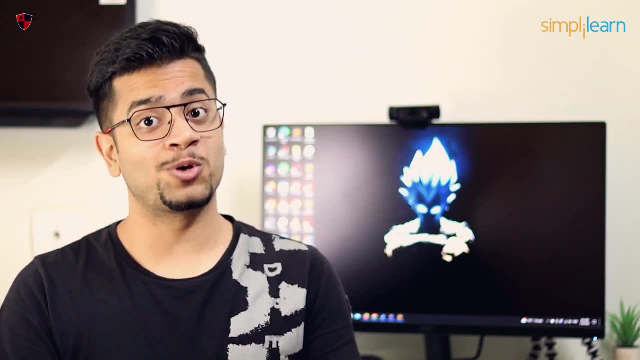 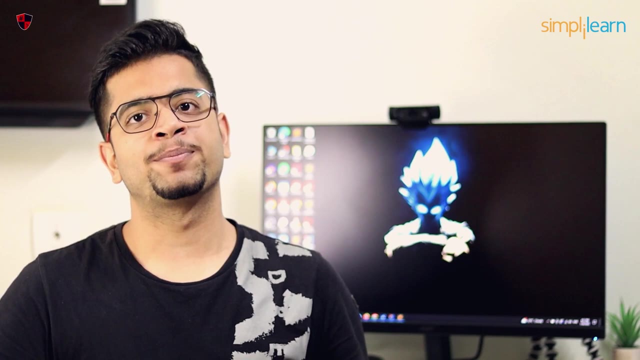 The fifth one is CISSP, or CISSP or Certified Information System Security Professional, And this is no doubt one of the best, Or maybe the best, The most prestigious certification in all of infosec earning, which you will be able to run complex security programs and manage them- just what CISOs and managers and directors. 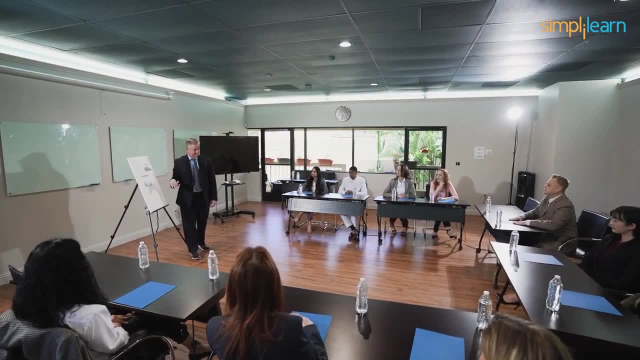 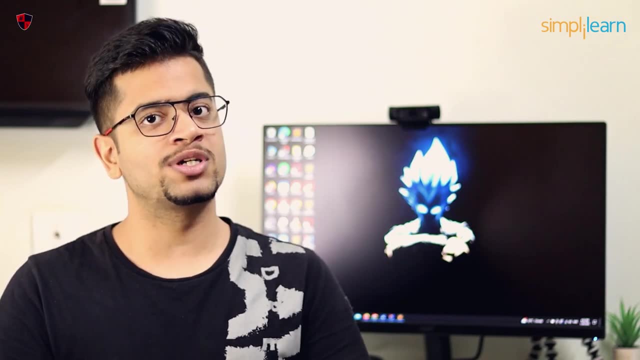 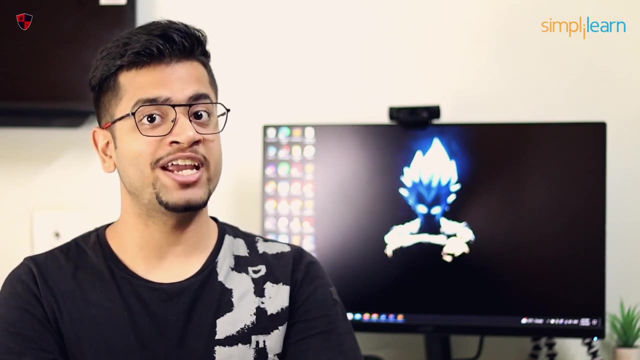 do, You will be capable of running a complete cybersecurity program, right from design, analysis, implementation and managing a complete infosec departments. that just not includes technical expertise, but also management expertise, because that's what you learn here And I can tell you the salaries here are way more than worth it. 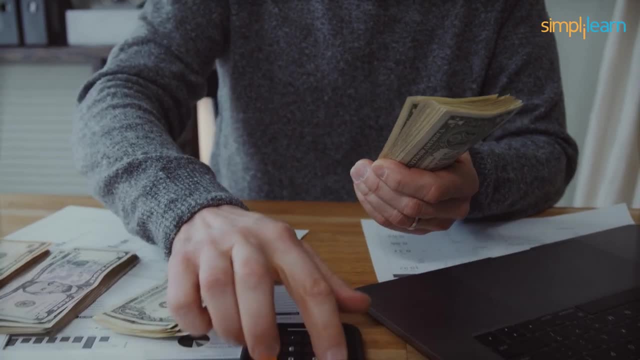 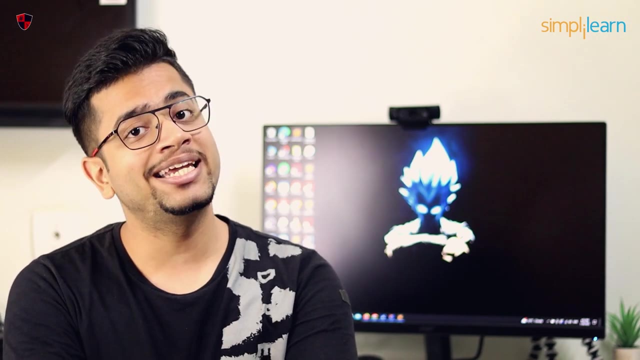 Seriously, it is meant for experienced professionals with at least five years of professional work experience in infosec and have a bachelor's degree. But here, if I talk about salaries, they can easily go to 50 LPA and even beyond 50 L for 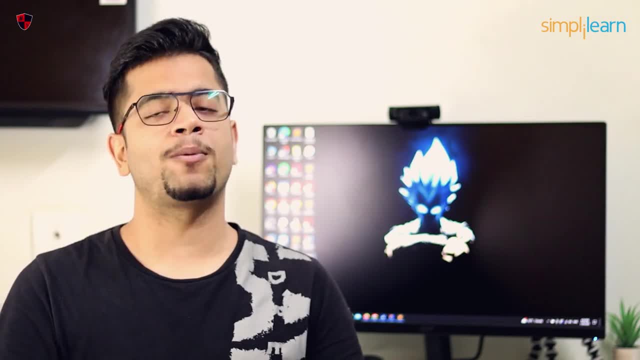 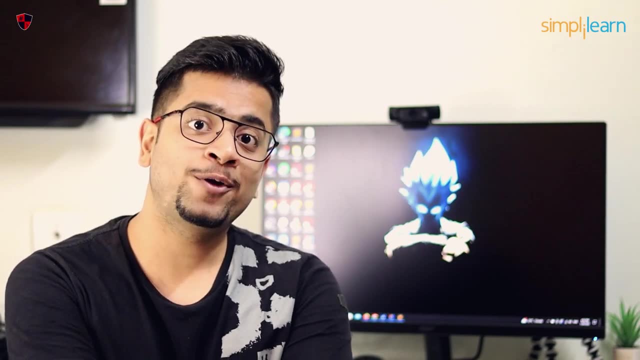 a CISO, And you can even work as a security consultant for world's top organizations, with a package only above competition. So these are my top picks for cybersecurity certifications in 2023 that you can do in order to get started in cybersecurity. Thank you. 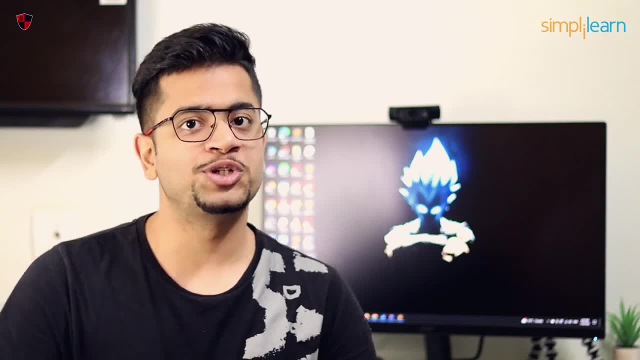 Thank you for joining me, Thank you for watching and I look forward to seeing you in the next episode of Cybersecurity Career, or even get eventually good and experienced and switch over to different fields if you are experienced. So I hope you like this video and you got something valuable to learn from this.